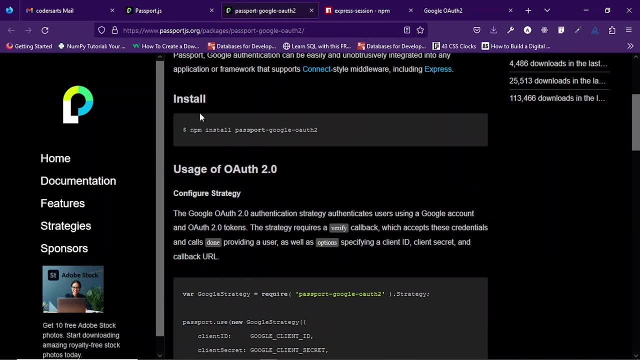 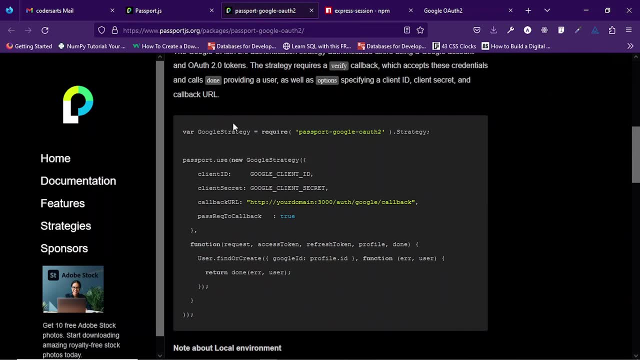 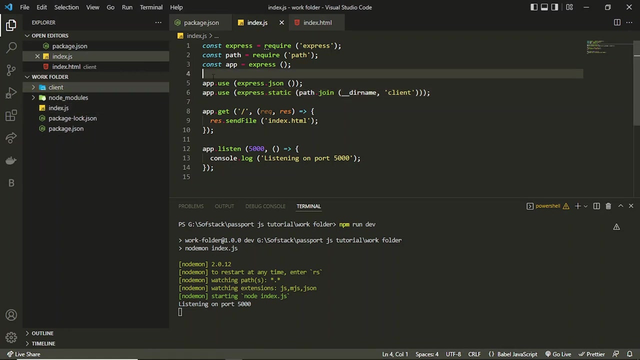 authentication. so you can see that it is saying you can install this passport, google oauth 2, which we have already done. and now it is saying you just need to do this kind of process. so you can simply copy this code here, or you can manually write if you want, and you can just paste it at the top, or you can create. 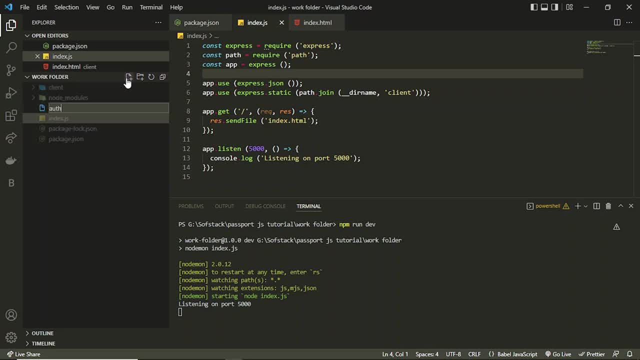 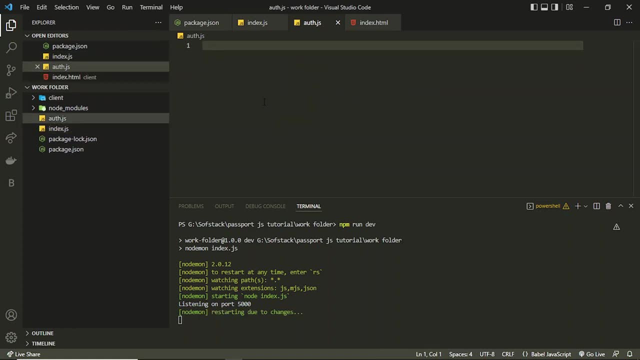 a separate file, if you want it to be clear from the other code. so i can create authjs file and inside that i can paste it. and we need to do some things here. let me just paste it once one more time. yeah, now we need to do some things here. 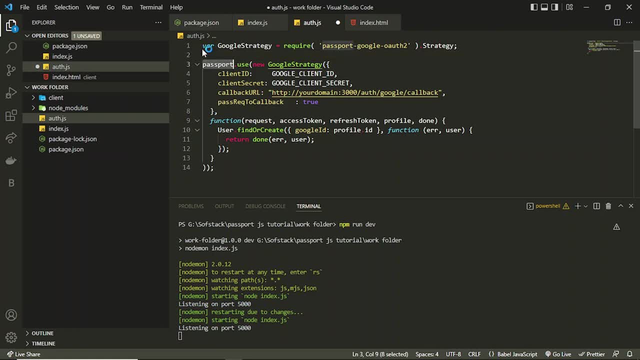 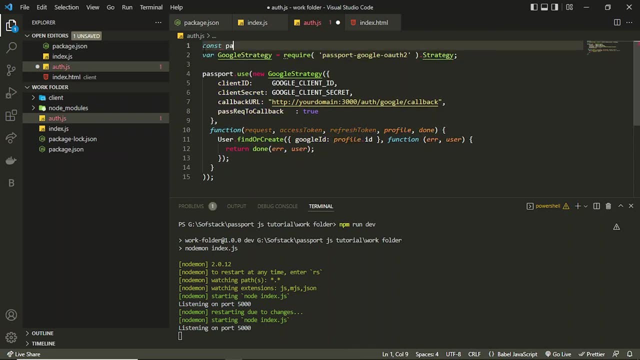 because passport is not initialized. so we can first of all import passport here. so passport is nothing but the passport package or the library which we have installed. we can just require it by saying: require passport. and now we can also make it constant variable, because we will not be using it twice. 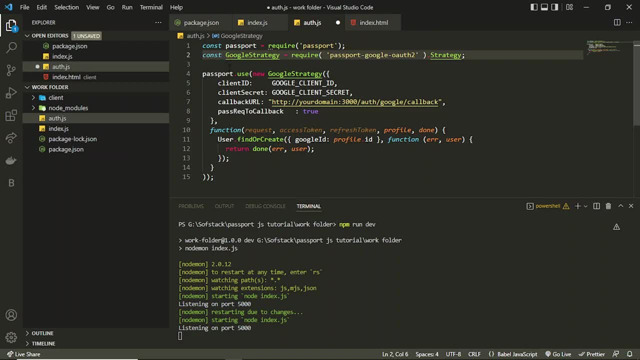 and then google says that we need to do some things here. so we need to do some things here, and then google says that we need to do some things here. we can also make it constant variable, because this strategy, this variable, will not be reinitializing it. 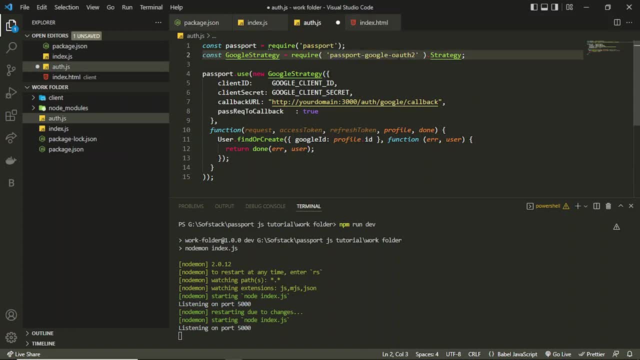 so we can make it constant. and now you can see, this is how it is creating this google strategy, and now we are using it in passportuse kind of middleware, and in which we are just creating a new google strategy in which we are passing our client id, which is google client id. 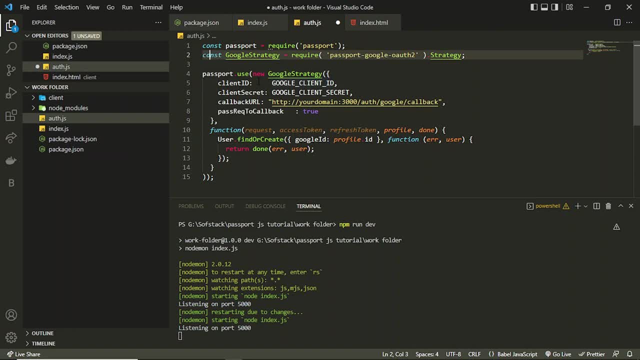 which will be getting from our google developer account. we are also getting client secret. so basically, we don't have these two variables: also the callback url which we need to create, and also after that there is a callback function which is here, in which we'll be getting all the information, such as the request we send: access token, refresh token. 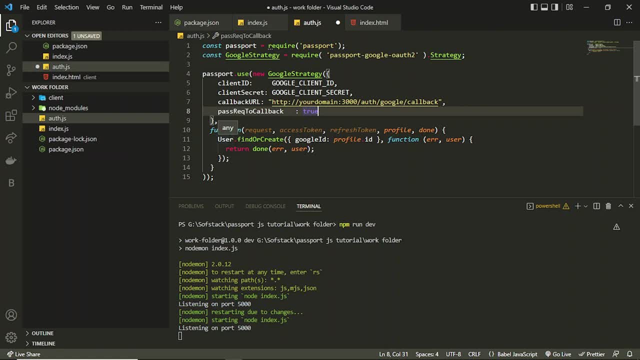 and the profile and the done function. basically, we don't want all these things uh like in which is available here, because it is actually creating, uh, the user and find, finding and creating the user from the backend database and updating the refresh token or setting up the google id to its profile. 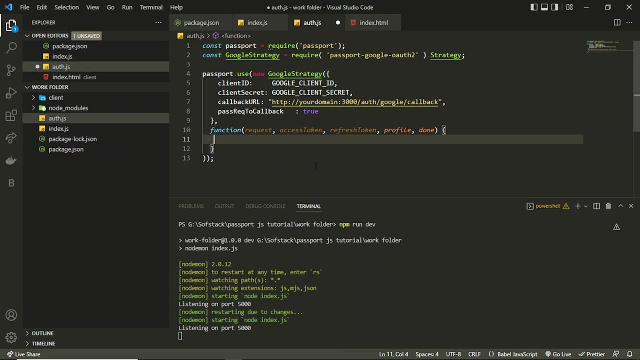 id. so basically, we don't want that because we don't have any database here. you can do this if you want, but we'll not be doing that. we are just returning the done function and the profile data, so we can just return this kind of information only. 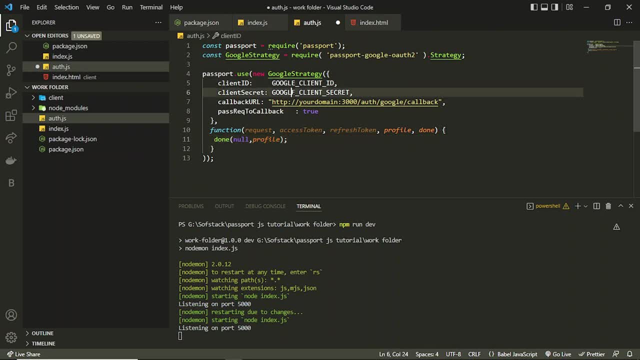 also for like implementing this google client and google client secret. we just need to first of all create an environment variable because we cannot store like secret information or like api key information or client secret kind of information in a normal page because that can be like visible to other users if 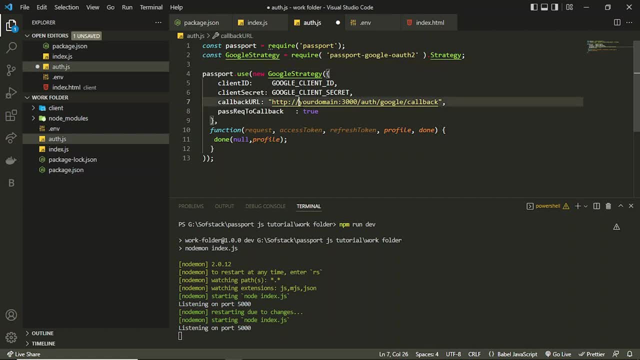 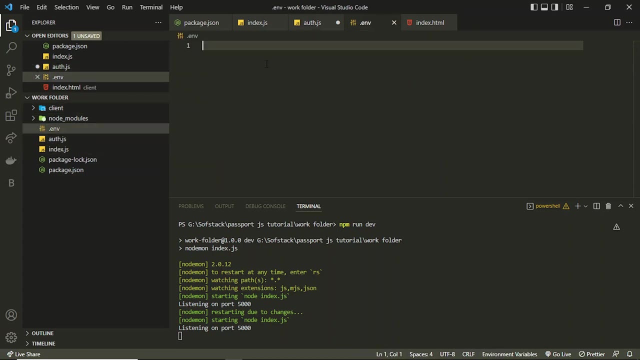 we upload this application into github. so if we deploy it in github, so that will be a problem if somebody sees this google client id and google client secret. so we always create that information or we separate that information from a normal javascript page or normal other pages. so we 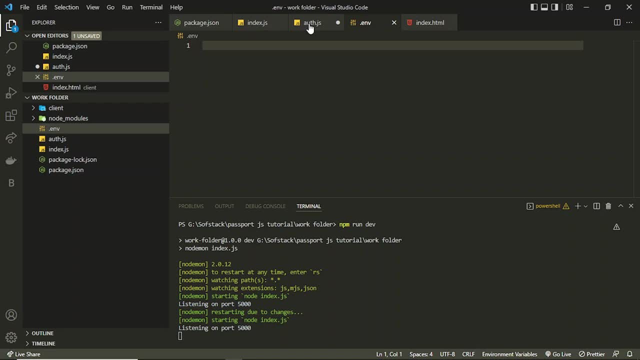 always set up in environment variables for that. so i'll be creating these two variables and for the data i'll be going into the developer account. so first let's initialize it and after that we have google client secret. we can copy that regularzoomenv right and to use environment variables. we have already installed the package. 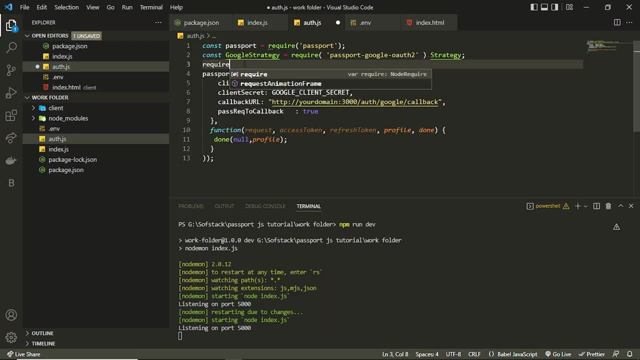 which is dot env. so we can require that package here which is dot env and we can call the method which is config. and now we can use process dot env here and we can call the method which is config and we can use process dot env here, similar for this: process dot env. process dot env now for the local host or like for the callback. 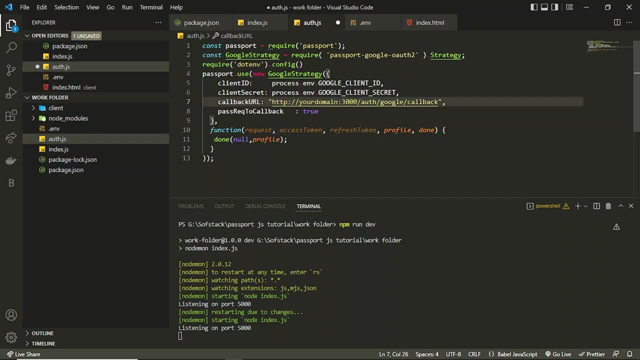 url like, it will be the url after like, which it will redirect to, after getting the information from the google, which page or which route will be the main callback url, so it will send the information to this route or it will be calling this route after making request from. 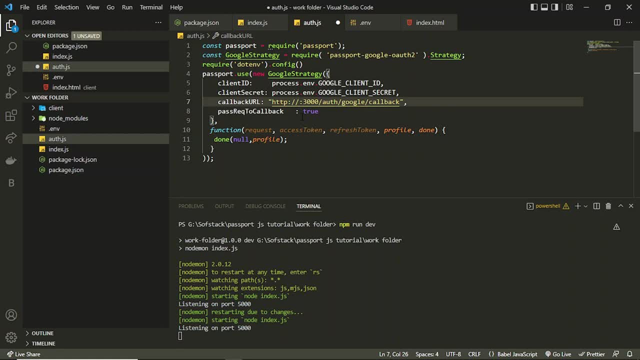 the google sign like authorization or authentication. after making the authentication, we can set up a local host- three thousand, not three thousand, it is five thousand- and we can set up this callback url like this: after making request from the google sign like authorization, back url in our like indexjs file. first let's get this google client id and google client secret. 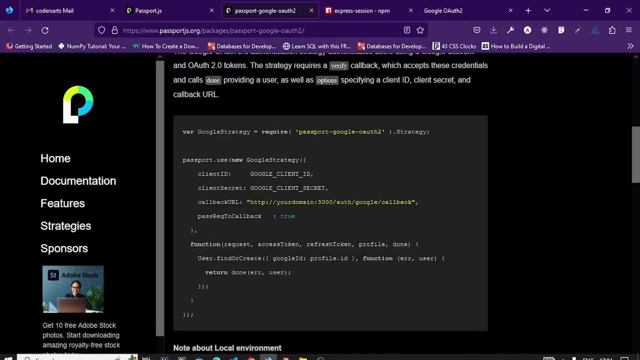 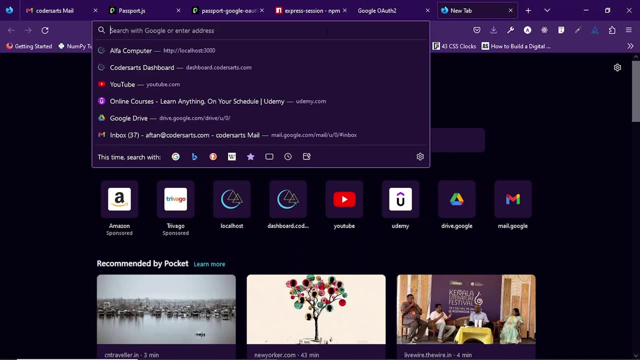 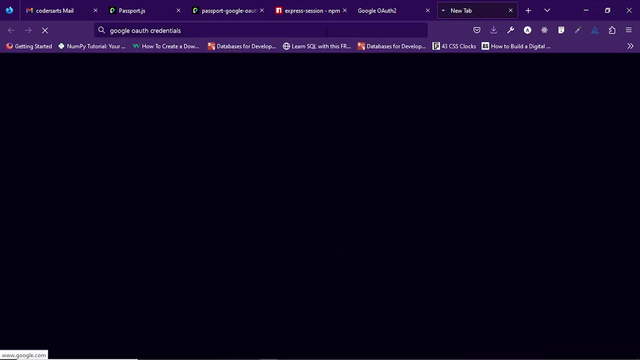 so first let me just go to the browser, and you can get that very easily. you just need to go to the google console or google developer console and create- create a google auth id. so for that i'll be just searching for google credential, auth credential, or you can just search for auth credentials. 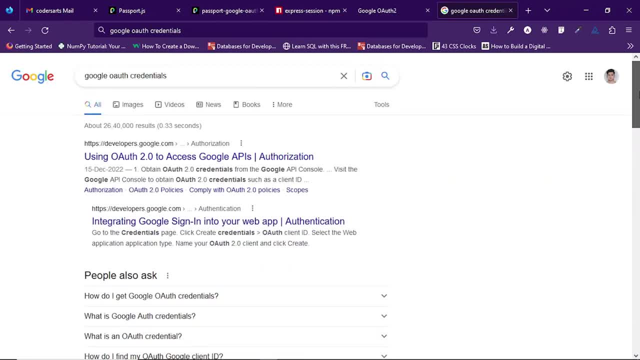 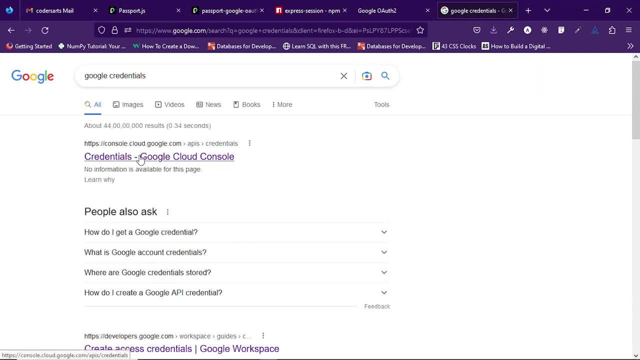 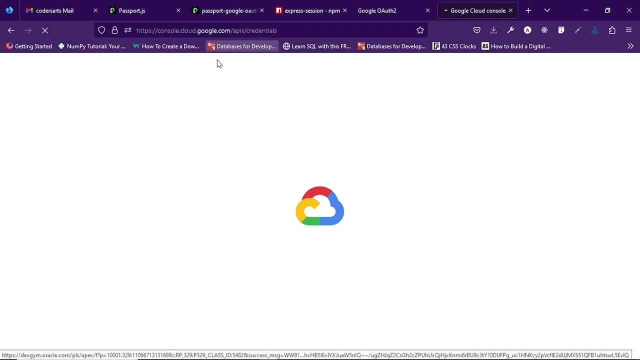 now the page will be: let's write google credentials here. simply, i can see it is telling me consolecloudgooglecom. this is our like main developer console in which, if you have already logged in, so it will show you the logged in screen and the credentials page where you can set up and create. 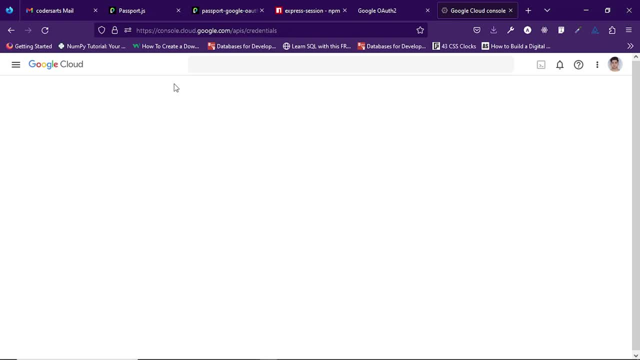 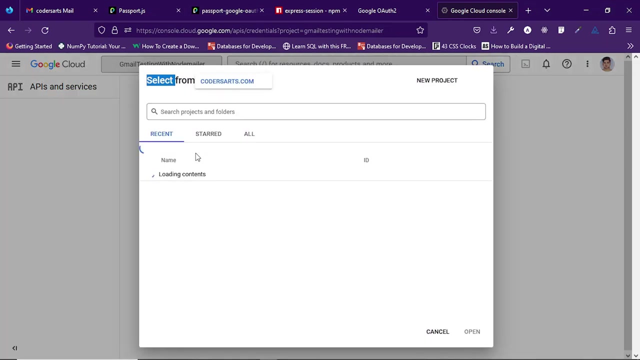 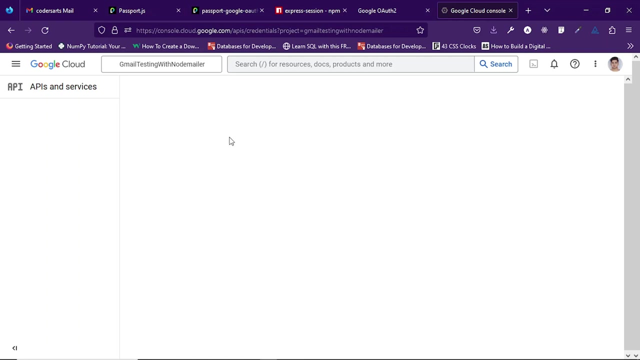 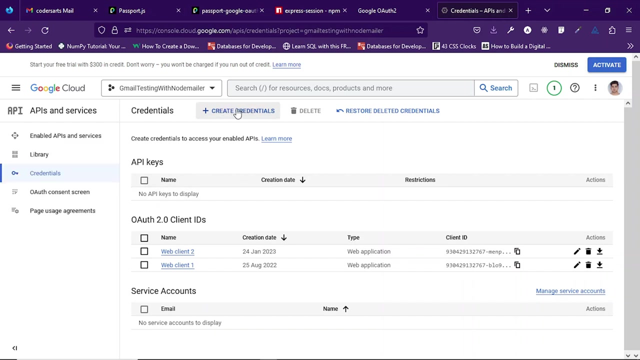 oauth api key. sorry, oauth client id and client secret for a particular project you have. so basically it will load. let me refresh it. let me clear it. you can see that we have this OAuth 2.0 client ID and client secret. I can also create one more credential here, so I have already created previous credentials. 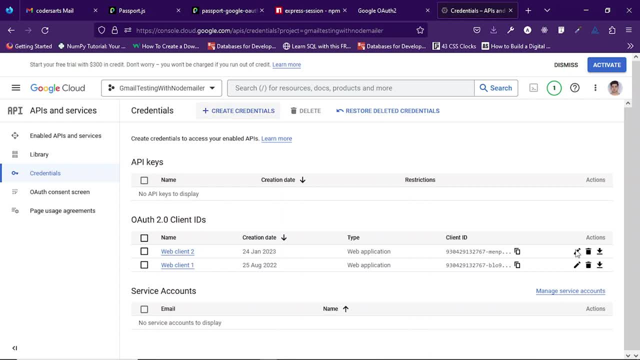 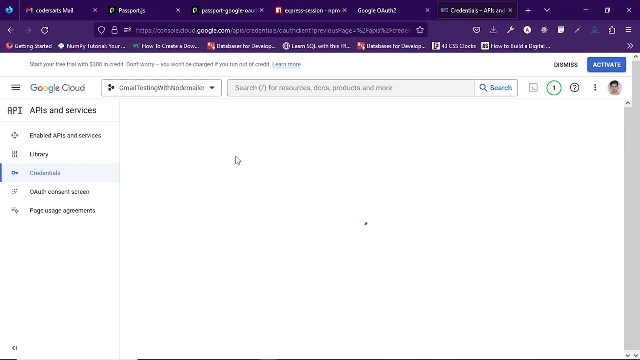 for like demo purposes. I can delete them like anyhow if I want. but let's just create one more credential by using create credential here, and if I click on OAuth client ID, it will jump to the next page where it will ask for some information that we can provide. now in here we can tell him what is the type of 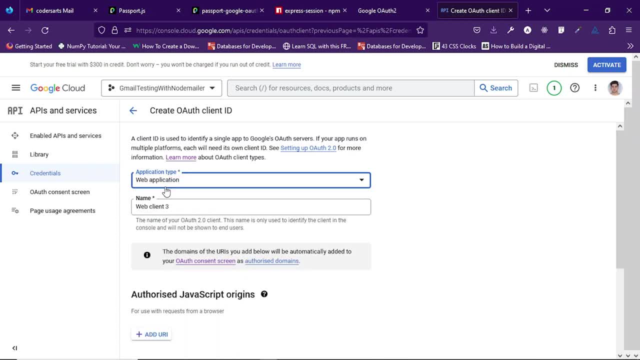 application we are using. we are creating it for the web application, so you can name it anything you want. let's let it be web client 3. you can name it anything you want. let's let it be web client 3. you can name it anything you want. let's let it be web client 3. 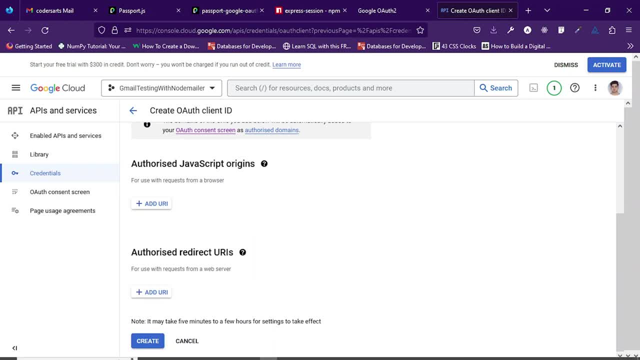 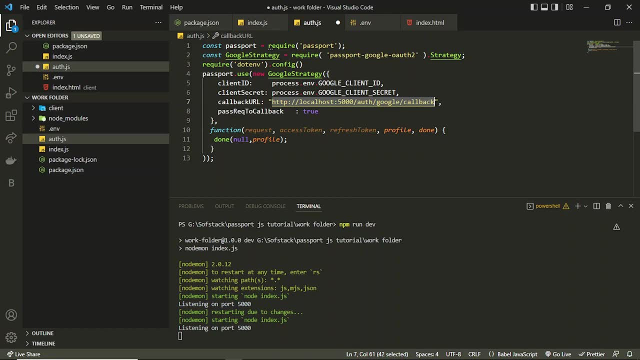 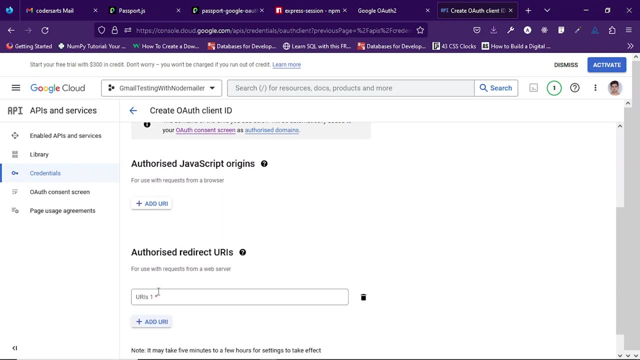 and we can also set up a redirection URI, which we have already set up here, so I can copy paste the same thing. so it will be the callback URL, so in which our callback will be presented after making the request from the Google. so I can create it now. so if I click on create and I can see that I have already created, 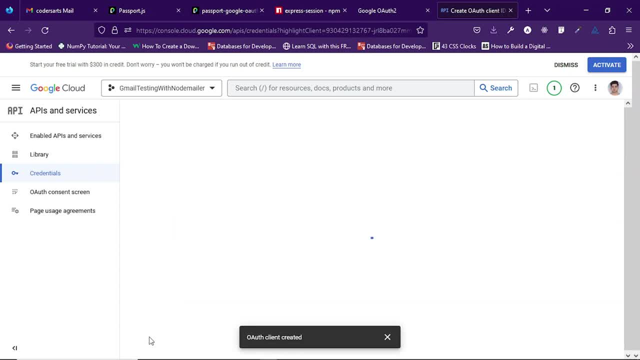 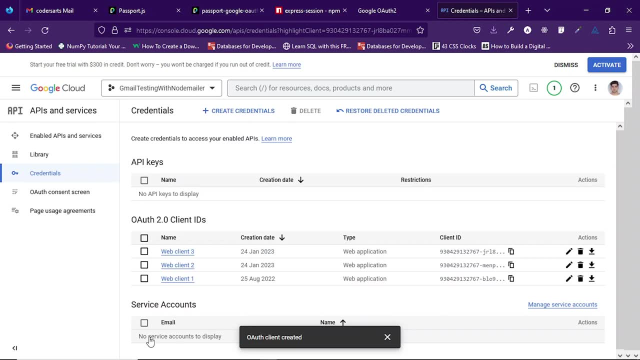 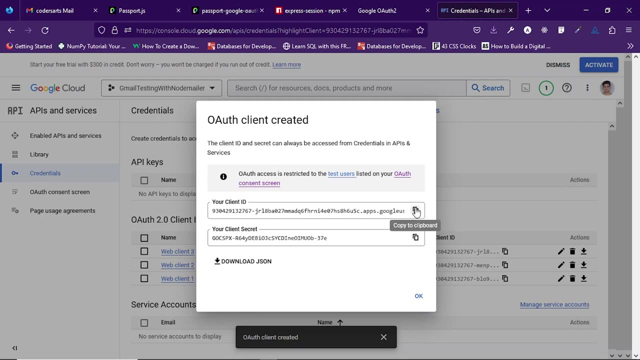 create this page or create this OAuth client ID. it will give me my client ID and client secret that I can store in my environment variables. so basically it will be for that. now I can see OAuth client created. now I can copy both these information and store it in my environment variable. so this is very 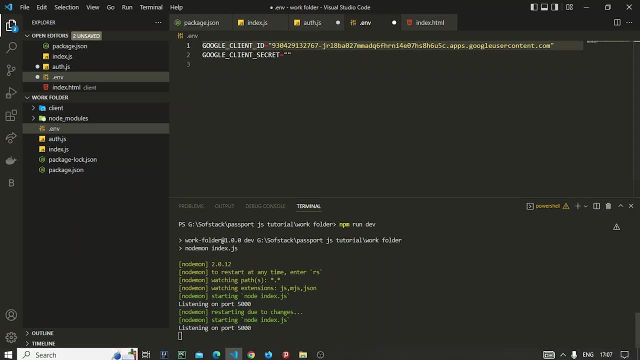 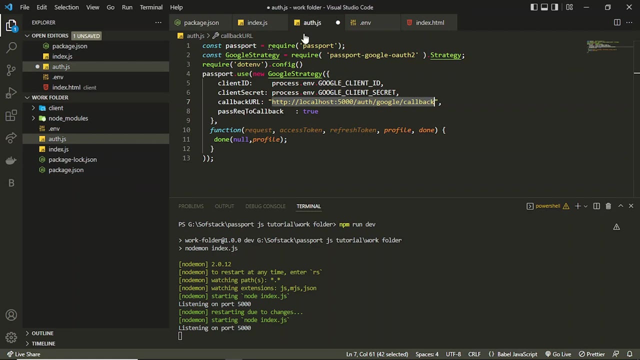 important step. you just have to forsake it and don't worry about it. I'm sure here in the video, but I will be deleting it after making this video. so this is it. we just needed that information from the Google. now, what we actually need is we. 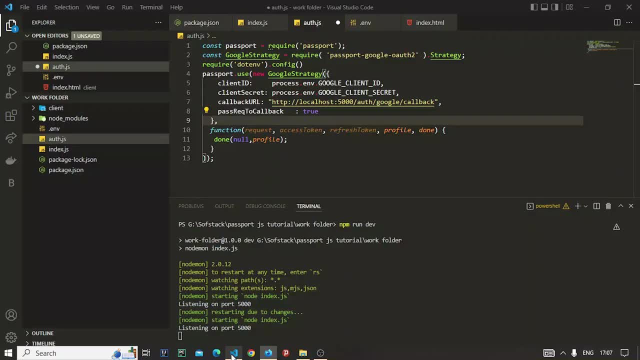 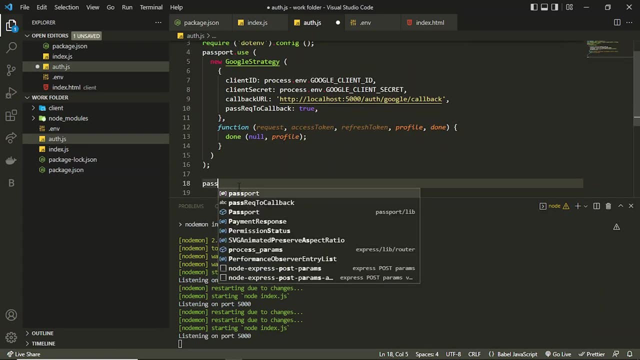 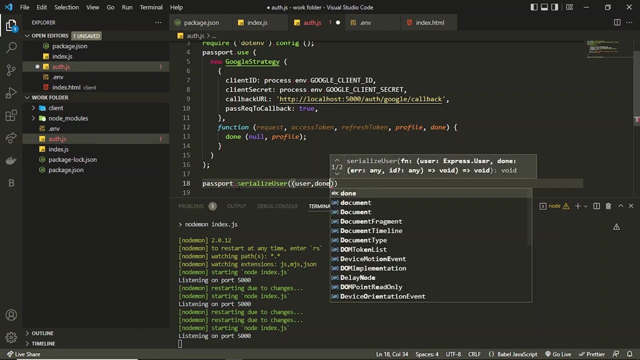 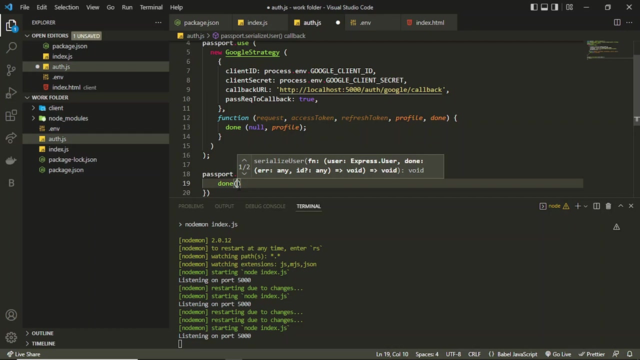 can press ok here and we can just save this file. so now we can also serialize the user by using passport dot serialize user and it will be a function in which we will be getting our user and also the method which is done and I can simply call the done method and initially the error will be null and the user will be. 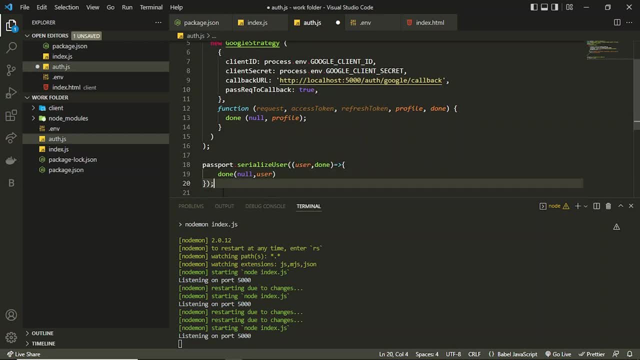 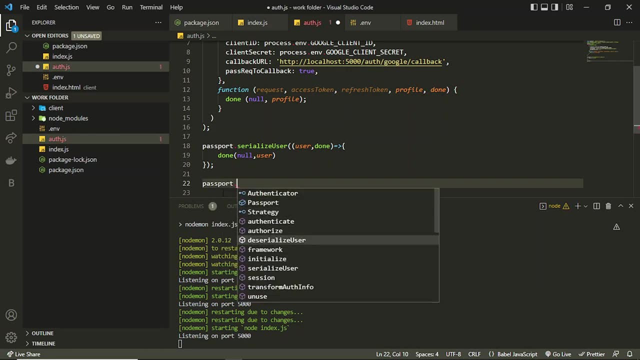 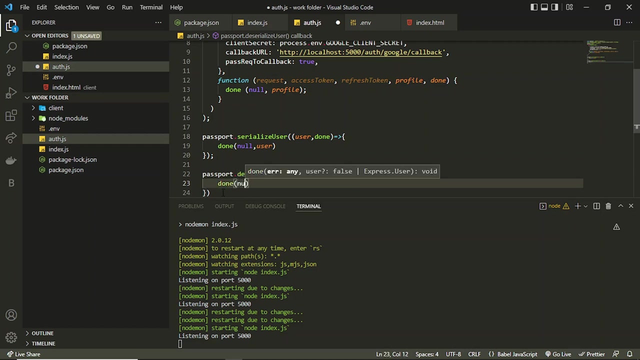 the user. so this we are doing for you- passportjs to like serialize the user, and similarly we can use deserialize if it is needed. similarly the same thing will go for them and I can call the done function again or done method again, comma and this user. so the auth page is: 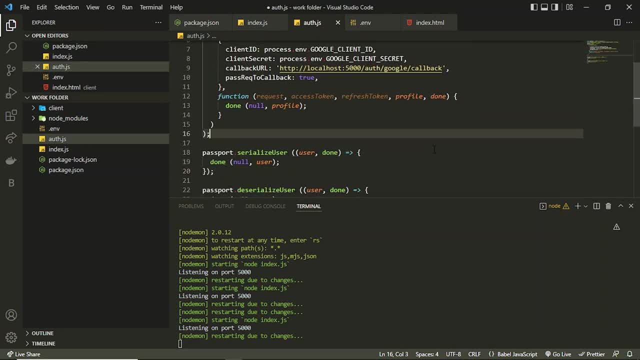 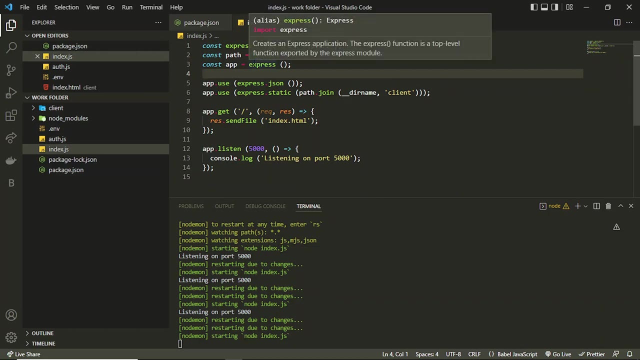 completed. now we need a callback function. we need to create a callback API or endpoint, which we have provided here. you can see that auth, Google callback, google callback. also we can require this authjs page here in this application. I can call it, require dot. backslash the page name: authjs, so auth. you can see. 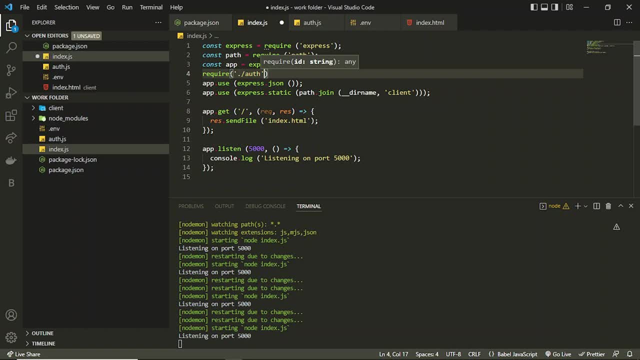 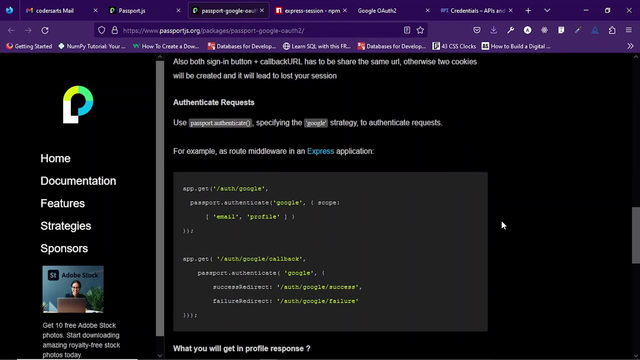 it is here. so we need to create a callback department which is called our. just simply write auth. it will automatically add js there, and if you go to the passport google auth screen in the next step, it is telling you that we just need to first set up this auth google. 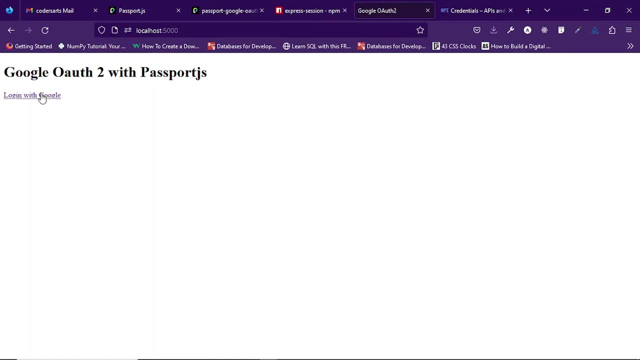 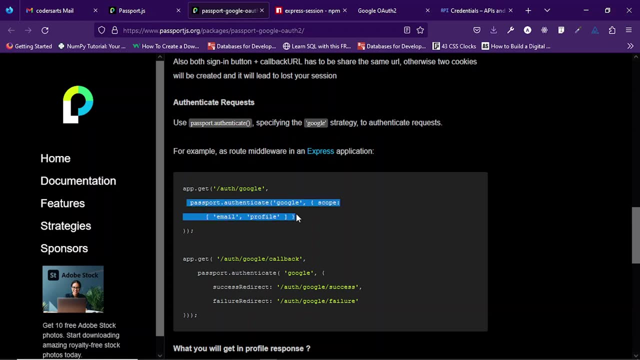 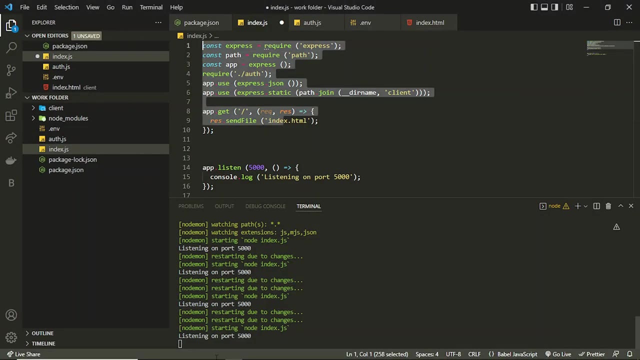 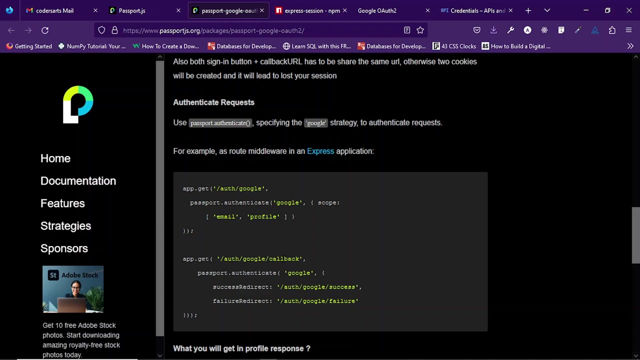 route, which will be the route when we click on this link, and after that, this passport authenticate will be called and this will actually authenticate it from this, like this page which we created just now, and after that it will send the response to this callback URL, which is this: auth Google. 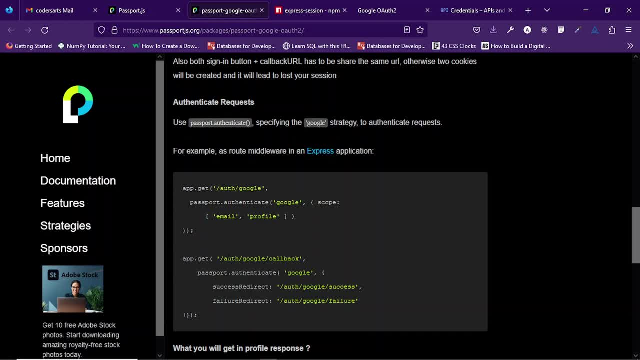 callback in which we can actually get the idea that whether we are authenticated successfully or not, so if you are successfully like authenticated, so we can redirect the user towards some page, and if you are not successfully redirected, so we can simply send them to a failure page. so we can copy this route here or this. 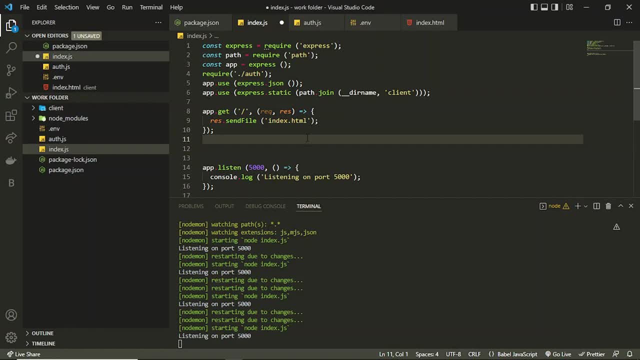 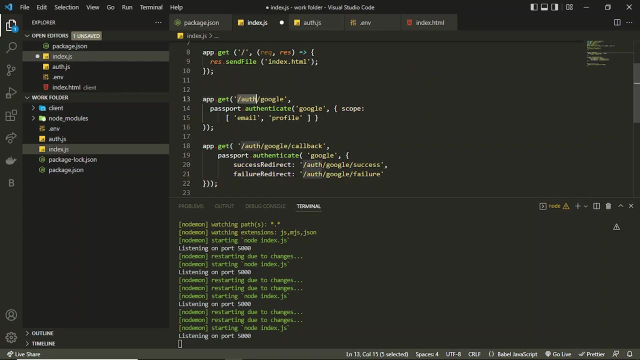 middleware or like express routes here, and I can paste them in here. make sure the naming which you are having here- auth slash- Google- matches with the indexjs href route. so make sure you're matching it. and in that we are simply authenticating with Google. this is necessary, you just have to. 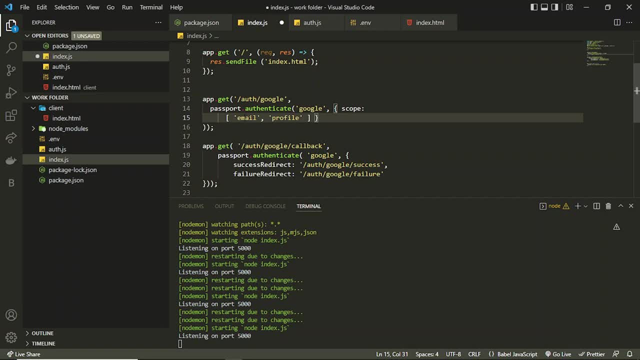 remember it, and after that we are simply limiting the scope to email and profile. so only these kind of information we will be getting, not every information from the Google account after the result. so you will be just getting the users email and the profile and then after that we are just. 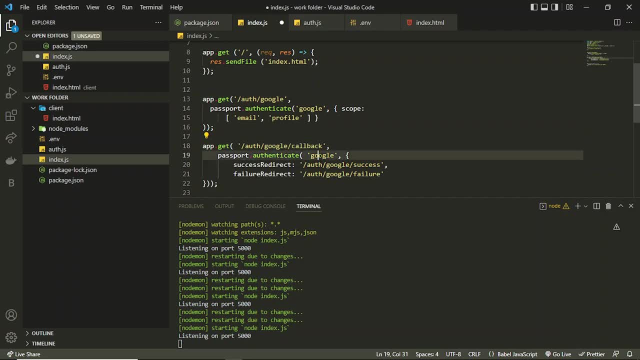 going into this Google callback endpoint. in this endpoint we are just checking we are authenticated successfully or not. if we are authenticated, so we are redirecting to this route, which is Google success, which we haven't created yet, and we can also create a Google failure route. so for both of 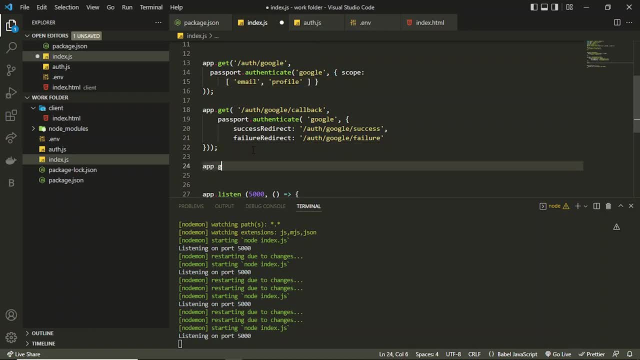 These routes we can simply use appget here. This was the route which you want the user to be shown. Let's say, I have this protected route so that I have shown you I have this auth protected. Then after that I can simply get the request and response. 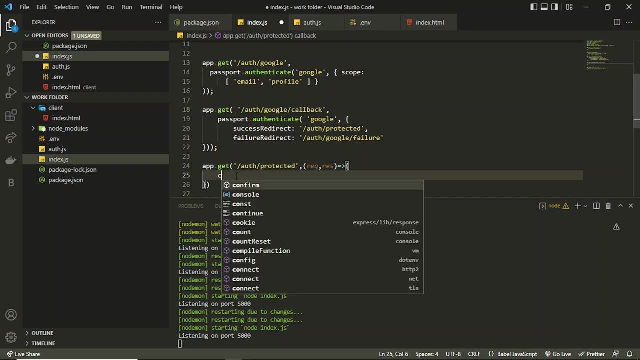 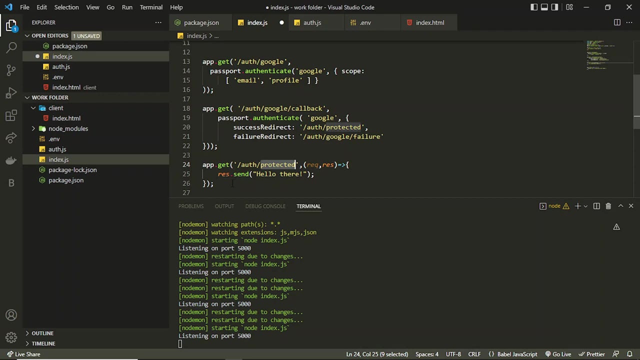 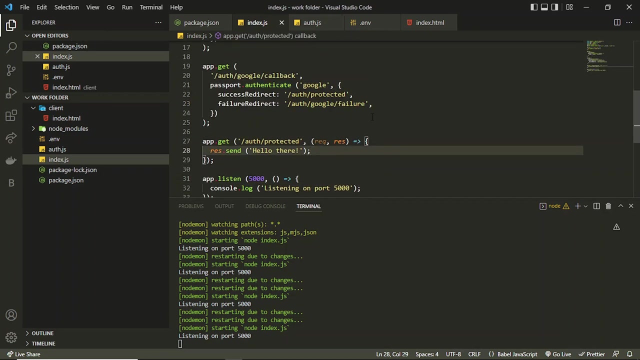 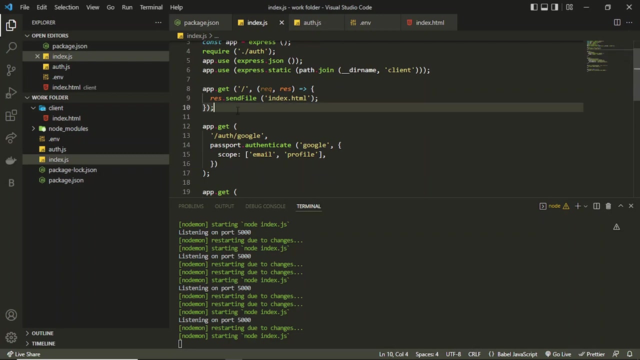 And simply I can send some data, let's say hello there. So this will be the protected route which will be passed After the successful login, So that we are creating here And simply, if I save this complete information And also we just need to set up some session tokens as well. 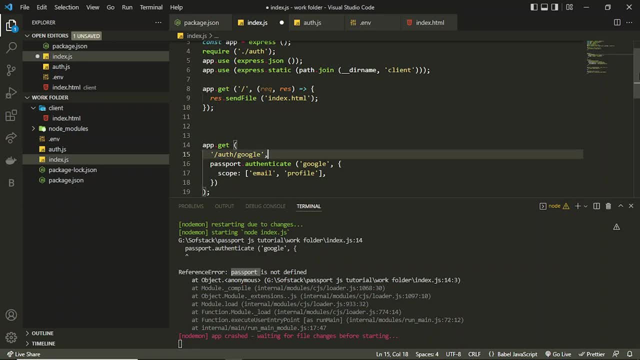 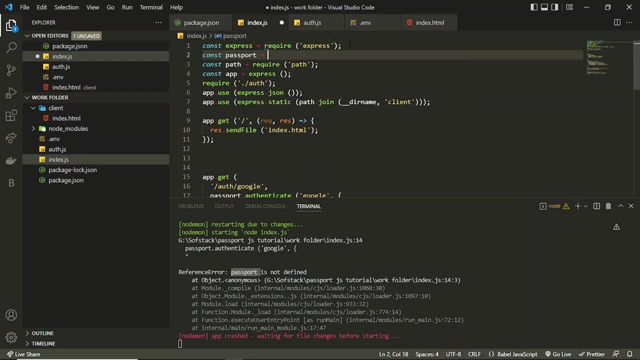 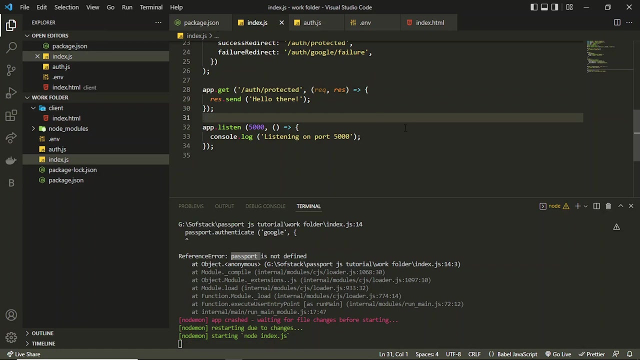 Now you can see, it is saying me: passport is not defined, So we can set up that as well, So I can set up passport again, passport, I can require passport, Passport here, Simply So. this is it, And also one more thing. we, one last thing we need to do is we just need to store all. 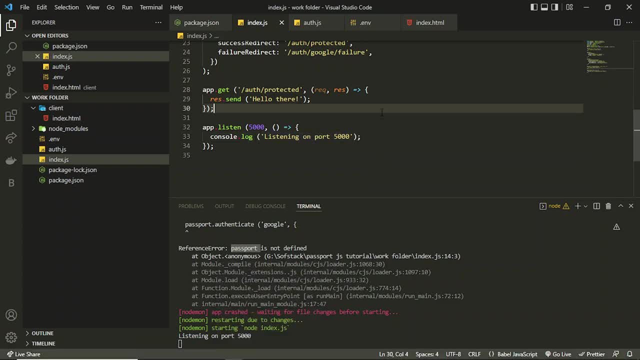 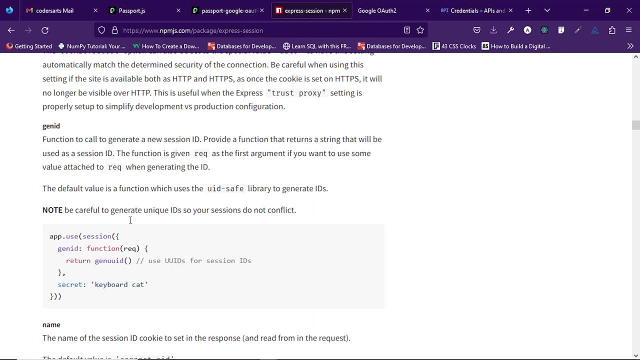 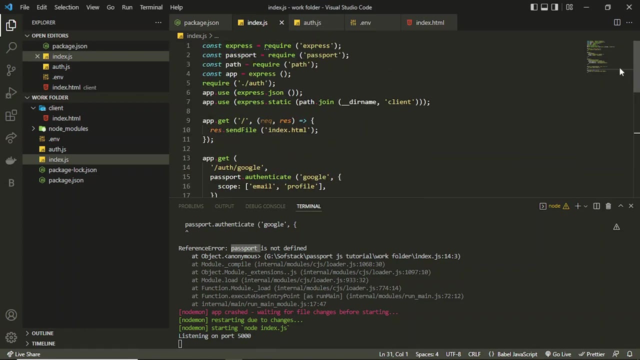 these information in a session token. So for that I'll be using, Okay, The express session package, which is a session management tool by express. So we can simply use express session and create the tokens or create the cookies. You can say simply: 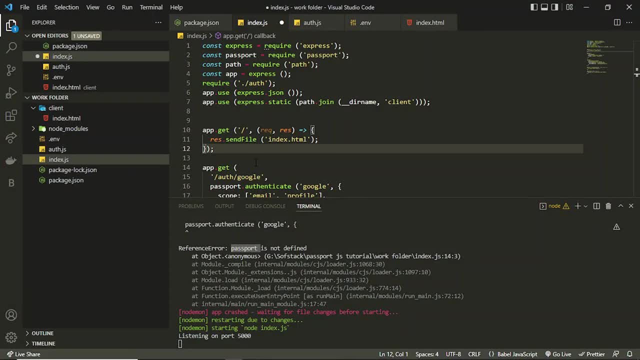 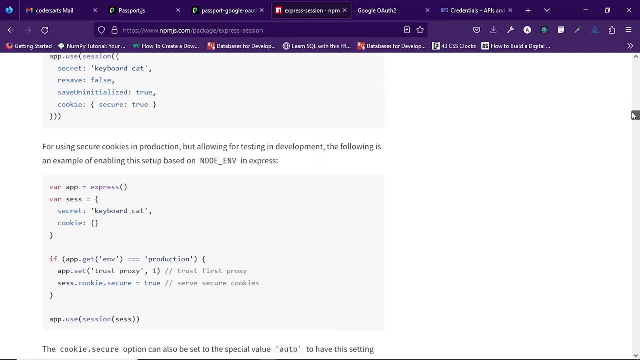 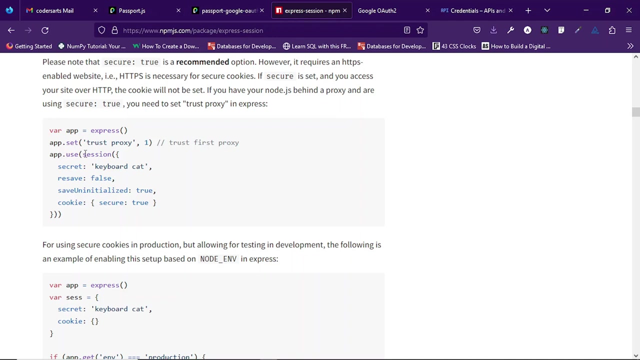 So for that I'll be just creating it with the help of appuse. first you can use it Appuse And inside that you will see that how you can implement it with. with this express session NPM page You can see it is using by appuse. 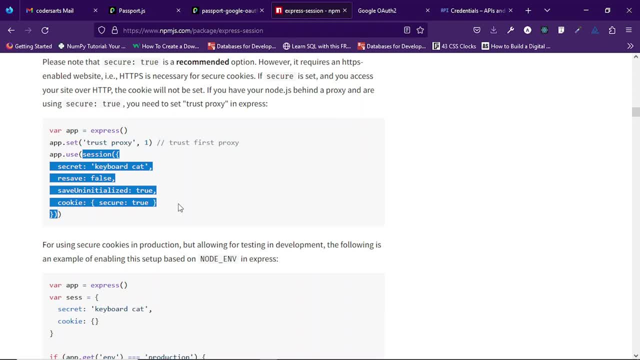 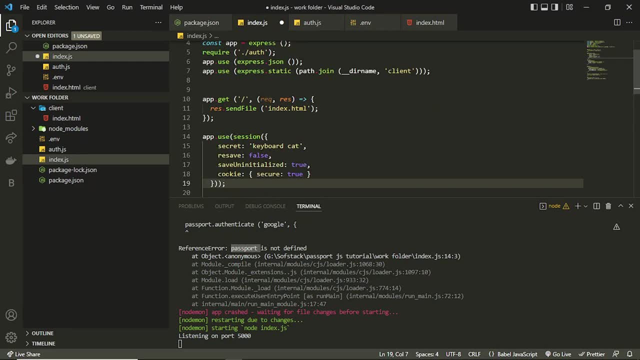 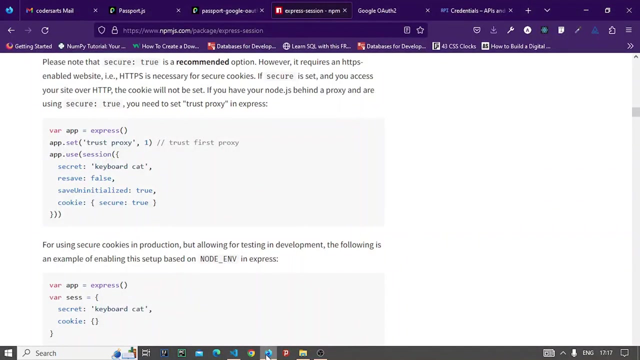 And then after that it is setting everything here. I can set up that here. Make sure you make it to false, Because if it is set to true, Then it means It will only create the session cookies whenever the like website is running on STTPS, not STTP. 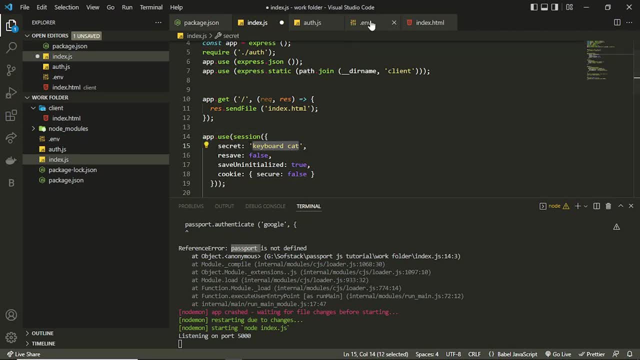 So you can change that. Also, this secret, you can store it in an environment variable. For now I'll be just using my secret or anything you want, So you can use it. Similarly, we can initialize, passportinitialize- Okay, Okay. 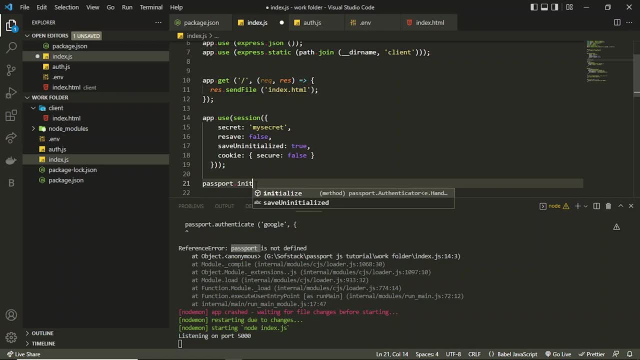 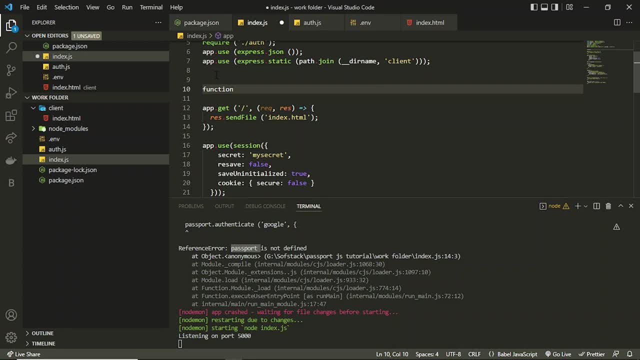 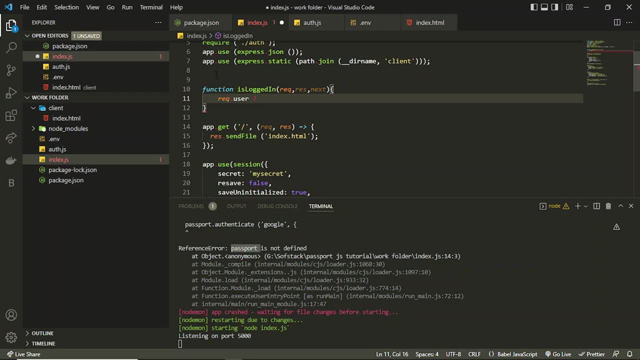 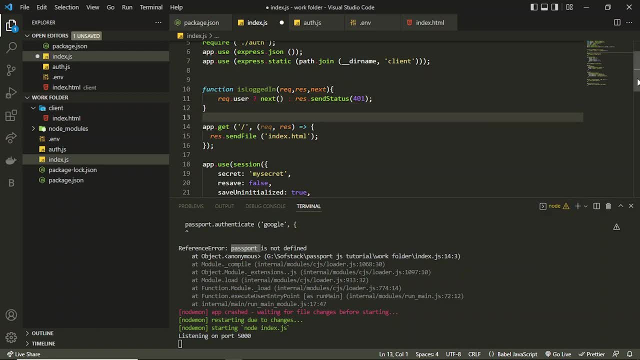 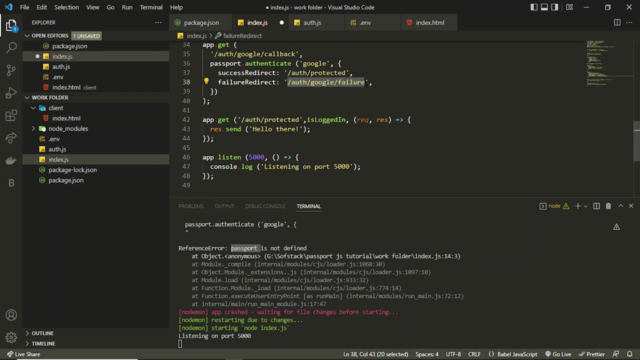 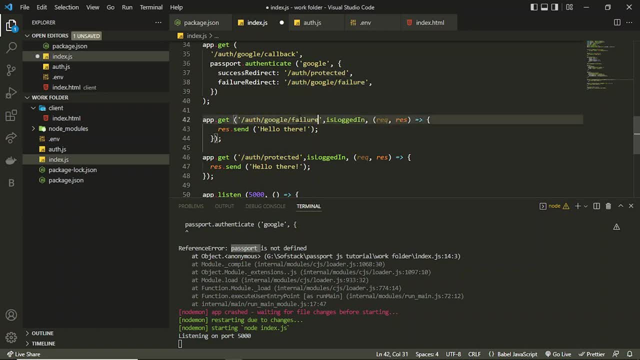 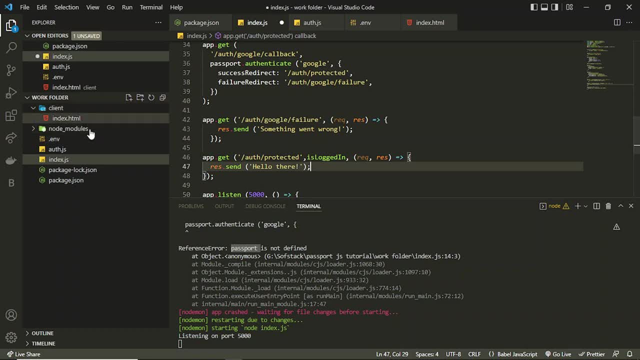 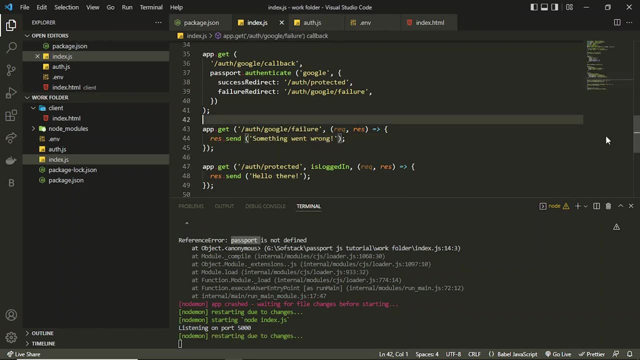 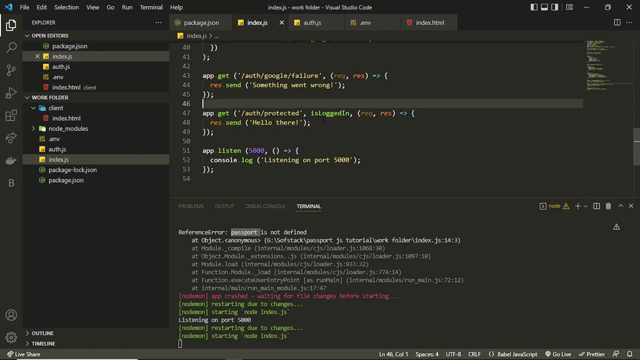 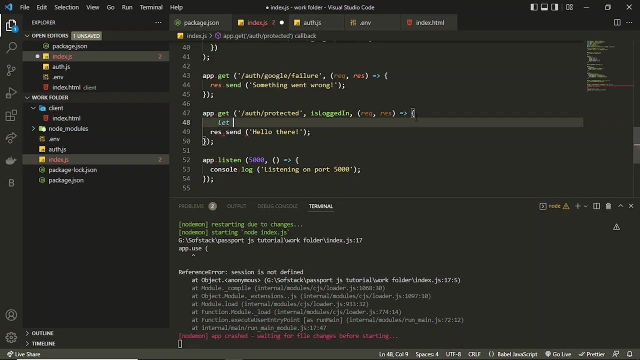 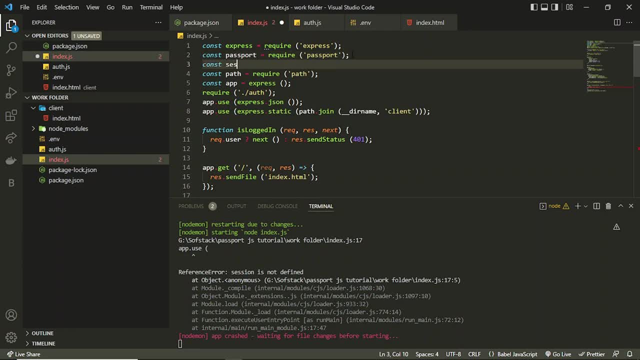 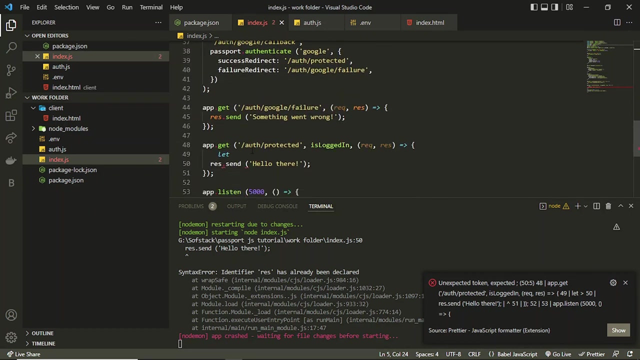 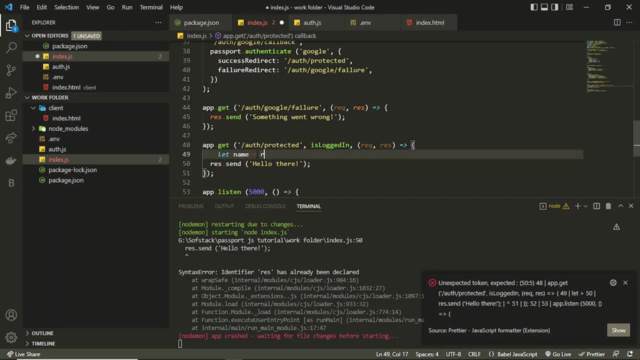 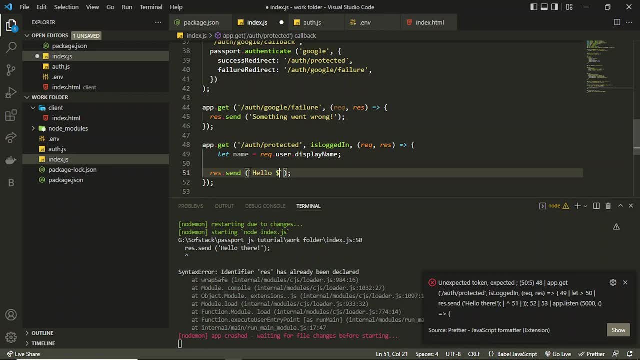 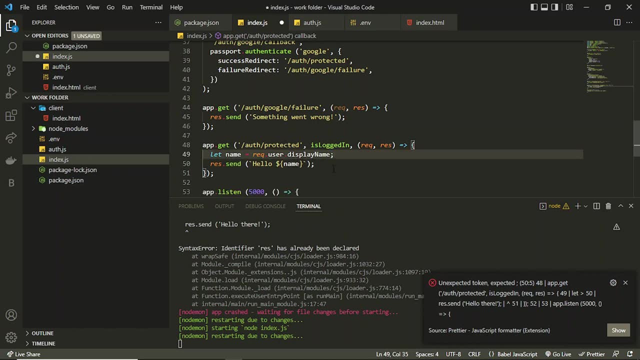 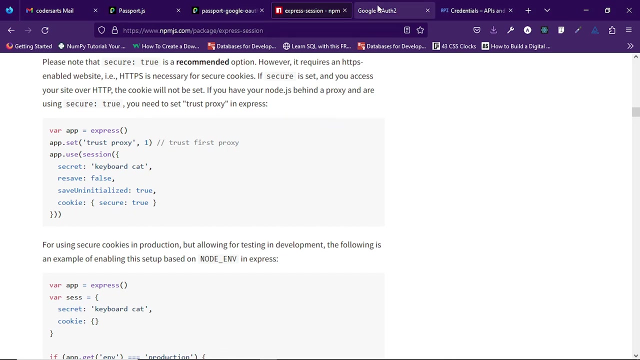 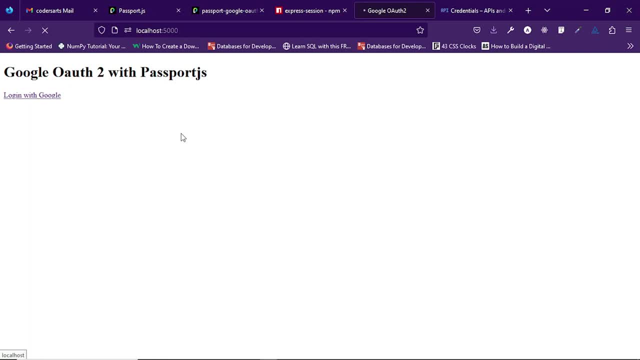 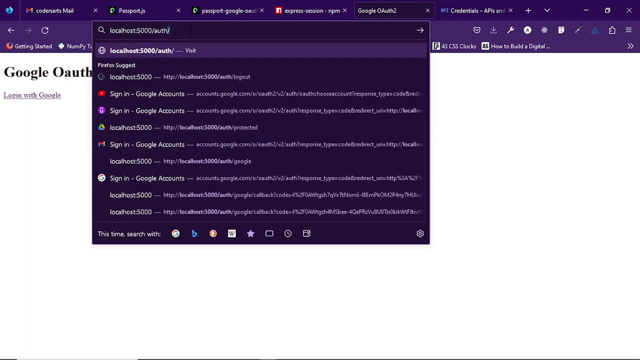 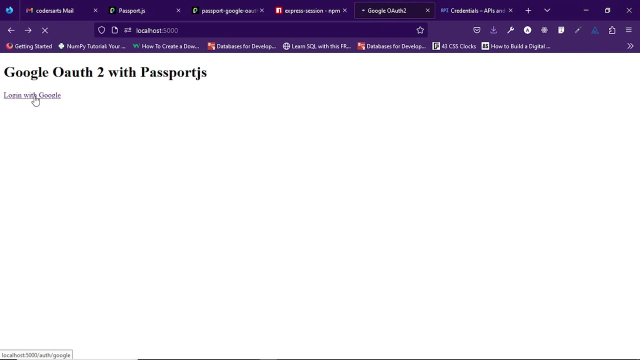 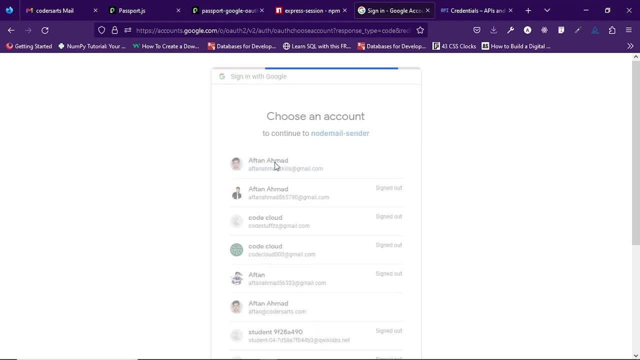 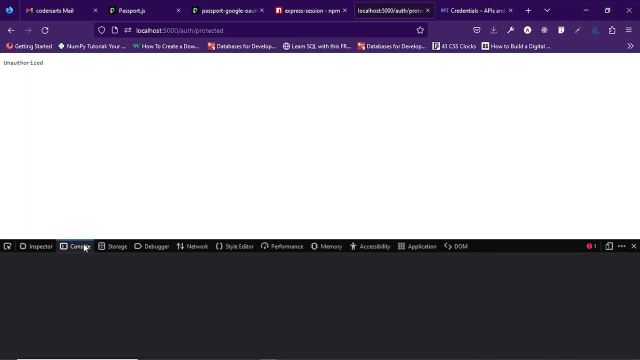 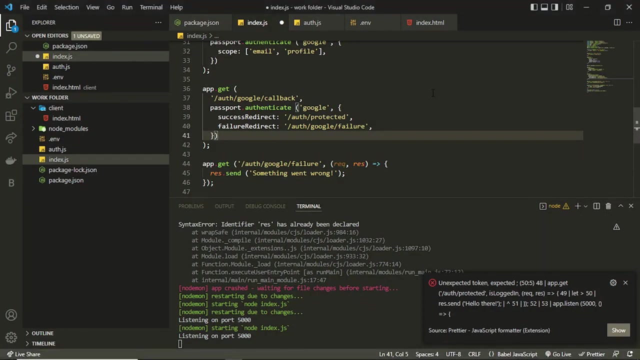 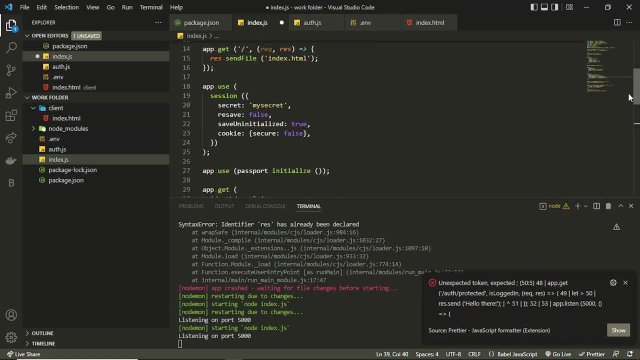 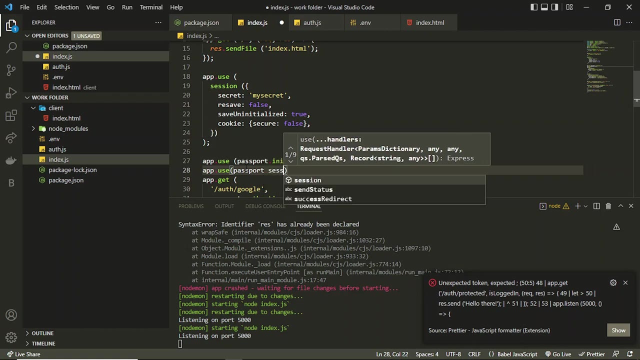 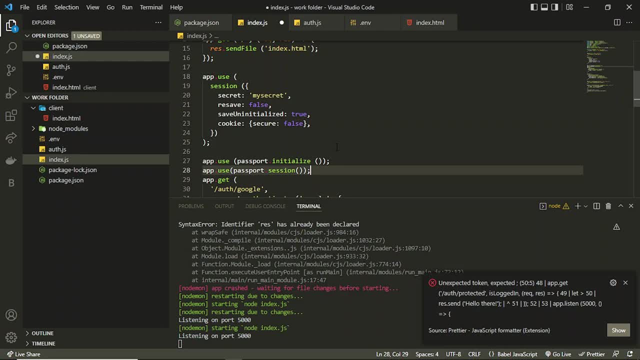 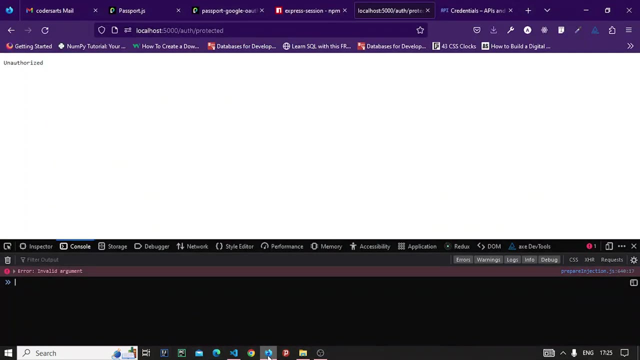 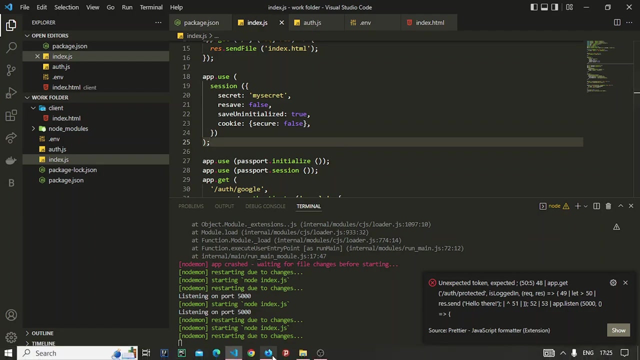 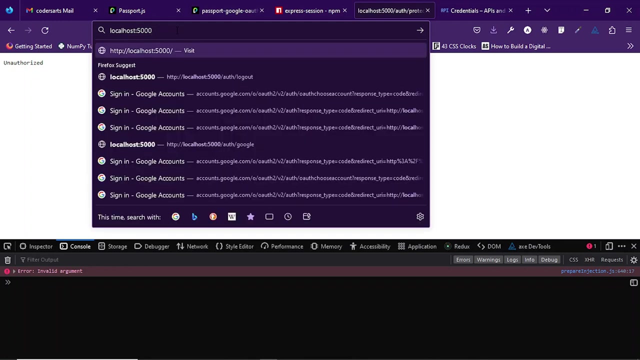 Okay, js to our session cookie. so this is. these three steps are very necessary. you have to remember this. now. if I save this file, that should work. now I can save it one more time. I can go to the main page, which is 5000. let's go to. 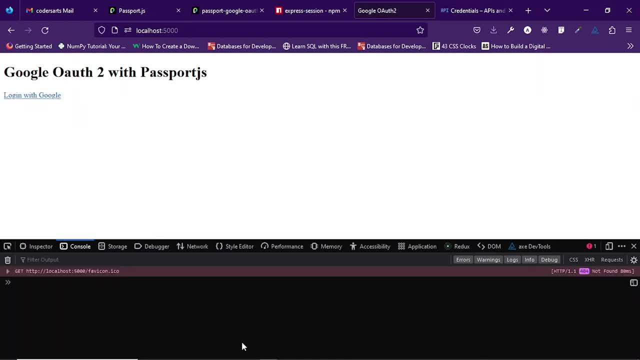 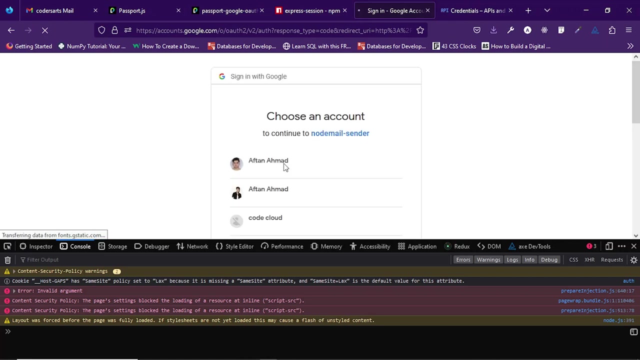 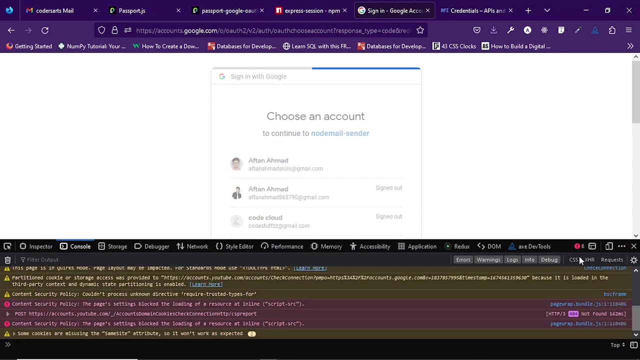 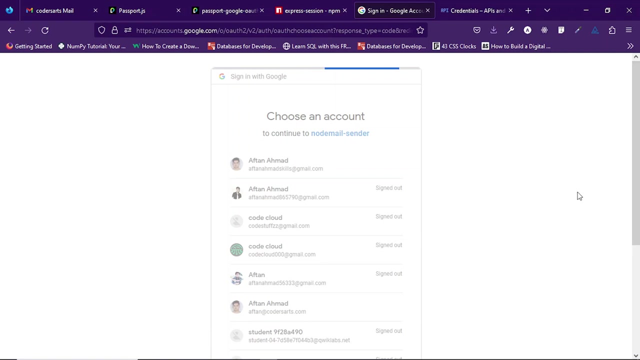 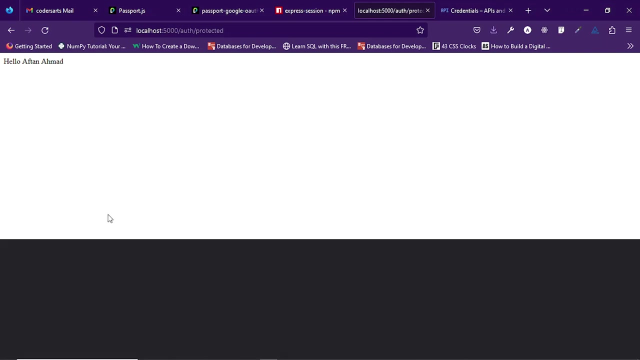 the 5000 page. right, let's log in one more time. you can see that it is showing me this page. let me just go with the first Gmail account I have. let me just close the console now. you can see that it is setting the data here and we are getting the cookies set. 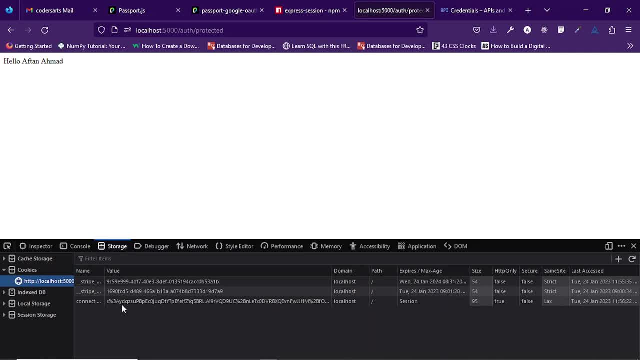 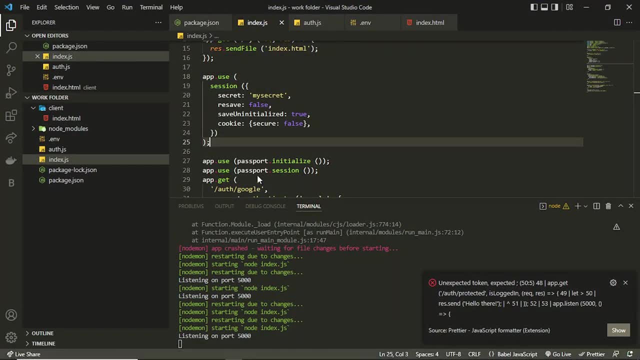 in the storage as well. so this is how you can set that, and, similarly, I can create a logout route, or I can simply delete it from my side as well. so these three steps are very important. you just have to know that these three steps are to remember it, to set the cookies properly, and now i can create a log out route as well.